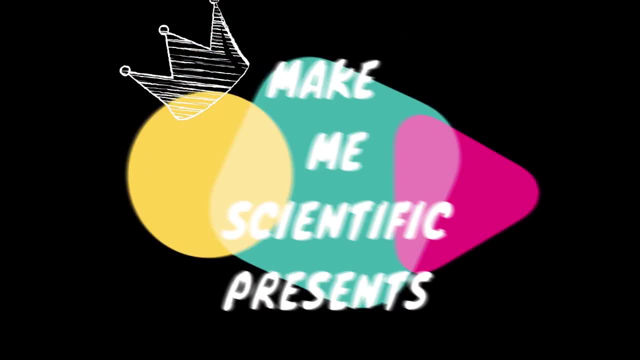 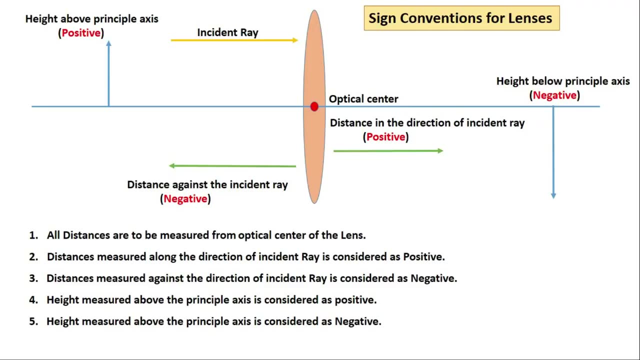 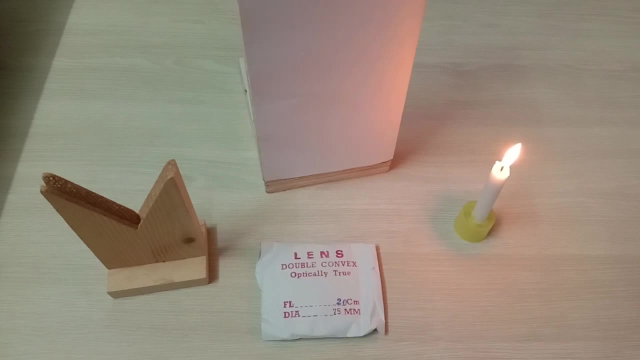 Hello scientific audience. so today I am going to perform a demonstration of image formation by convex lens and this is a very useful demonstration for the students from grade 8 to grade 12. for this experiment I have taken a lens- convex lens- of focal length 20 centimeters. you can take the convex. 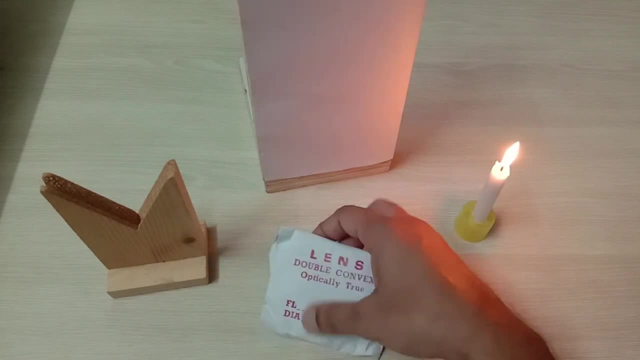 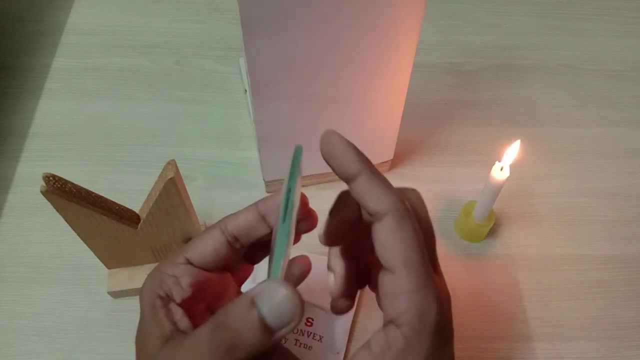 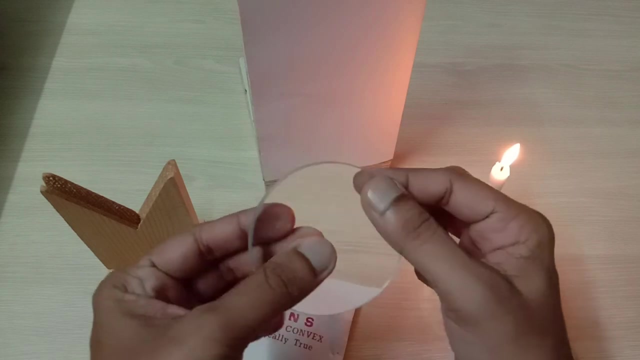 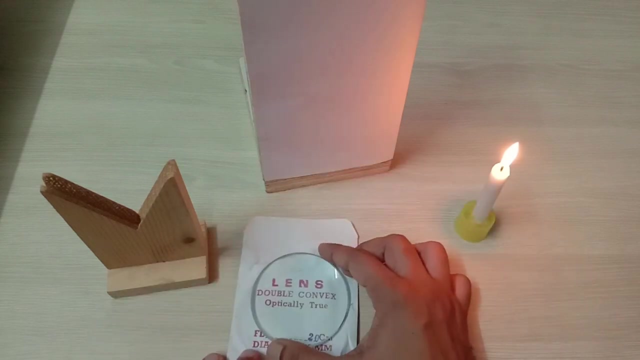 lens of other focal length also, you can see that the convex lens is thick at the center part and as you go towards the edges it becomes thin. a stand or a lens holder, a screen which is a white background, a candle mounted on a plastic cap which behaves as our object. 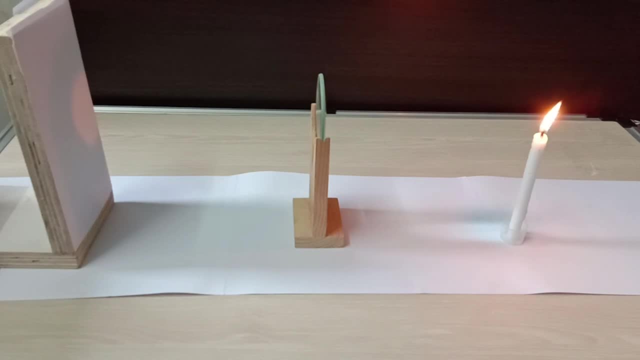 this is our basic setup, guys, so I am going to show you how to make a convex lens of focal length 20 centimeters. I have taken few a4 size paper on which I have arranged the lens, the candle and the screen as follows. I can move the lens towards the candle or away from the. 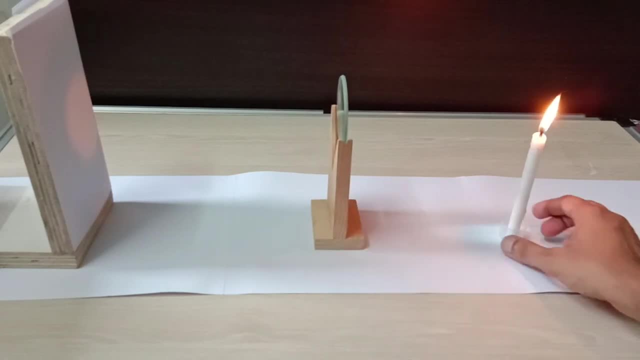 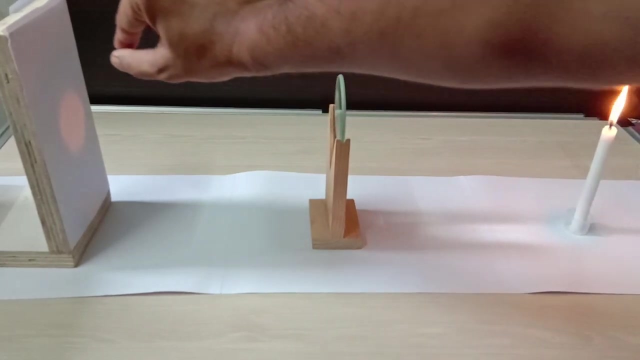 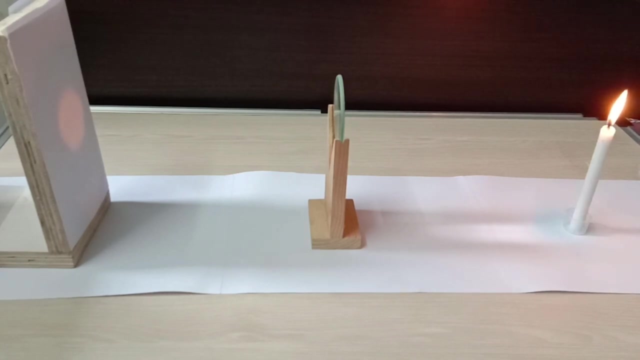 candle. even I can move the candle towards the lens or away from the lens. the light rays coming from the candle will fall on the lens and since the lens is converging, it is going to converge the rays on the screen to obtain the image. if the image would be real, we will be. 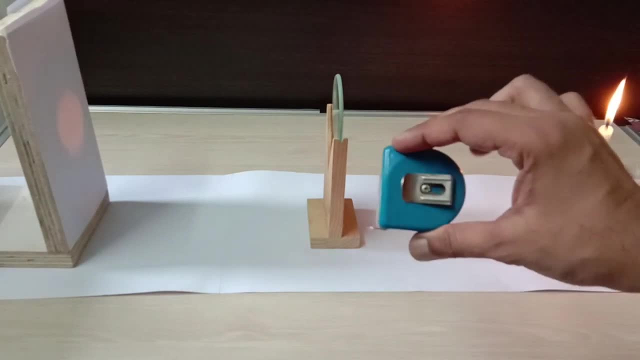 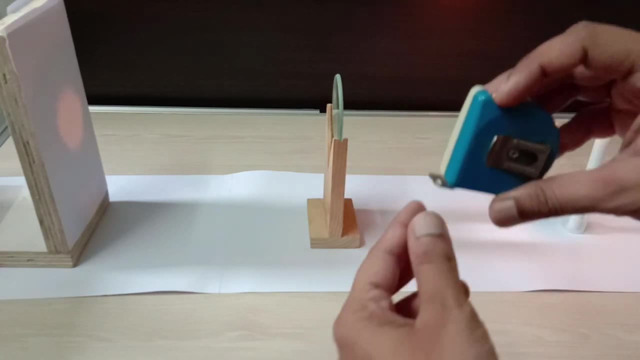 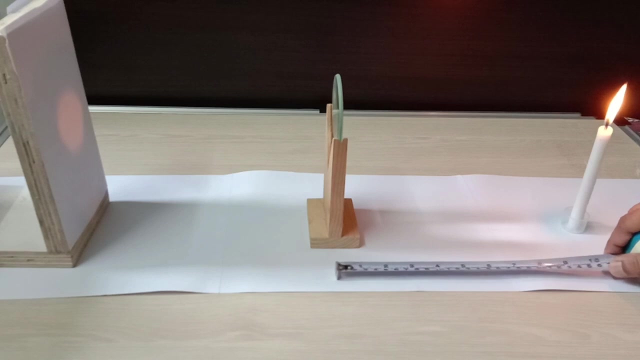 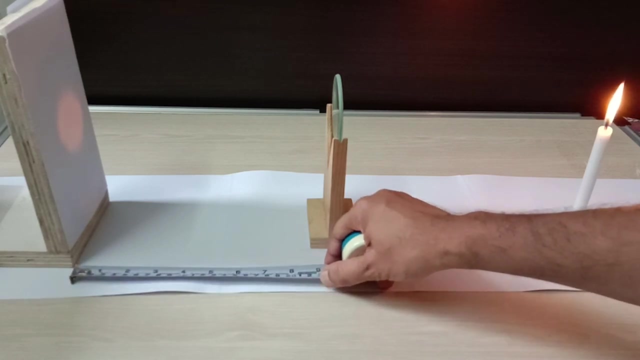 able to see it on the screen. I prefer measuring tape over scale to measure the distances: the distance from the candle to the light ray and the distance from the light ray is. the distance to the light ray to the lens will be our object distance and the distance from the screen to the lens would be our image distance. 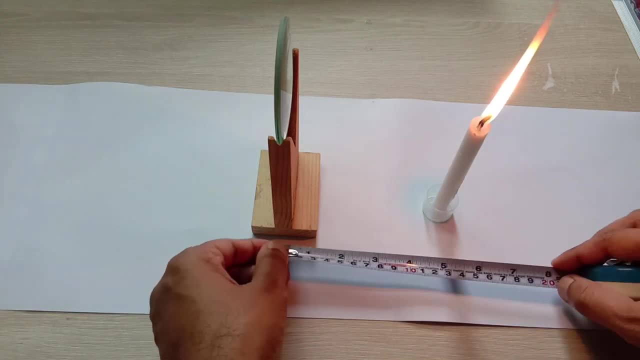 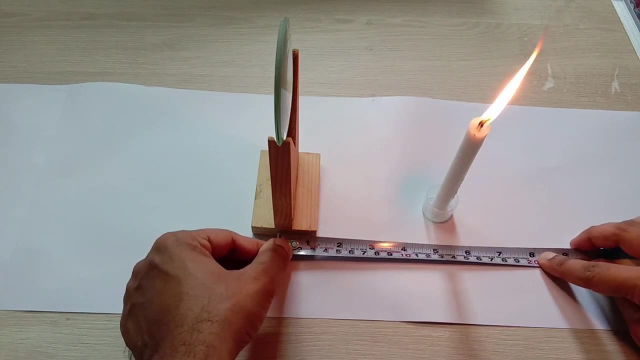 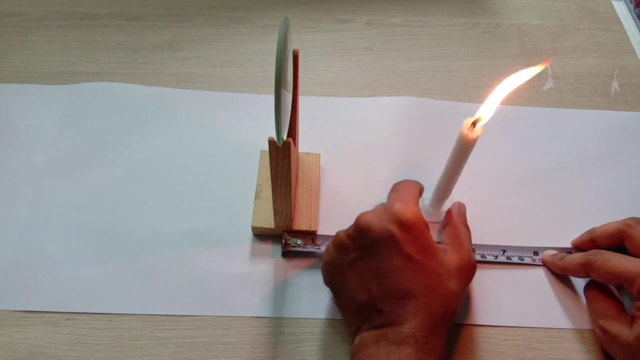 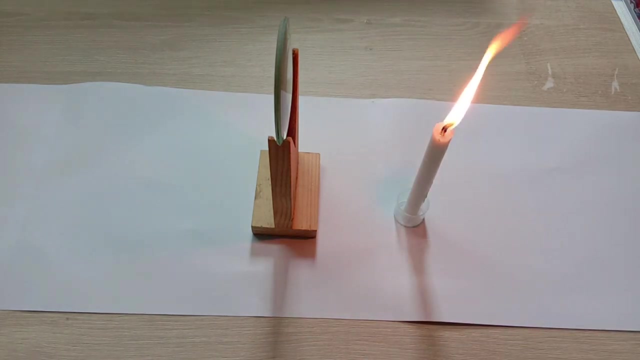 here i have arranged the object, or the candle, at a distance of 10 centimeters from the lens, so the object is between f and o, because the focus is 20 centimeters far away from the lens. so we should be getting a virtual image which we will not see in the video. 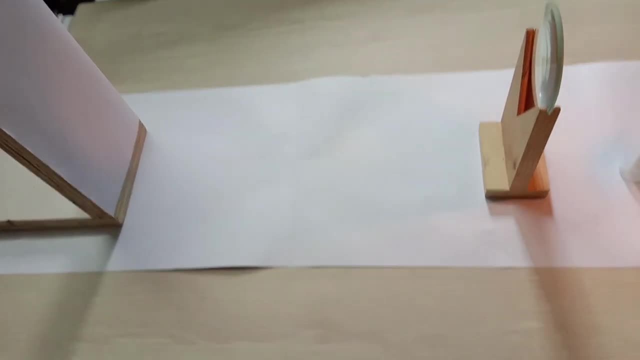 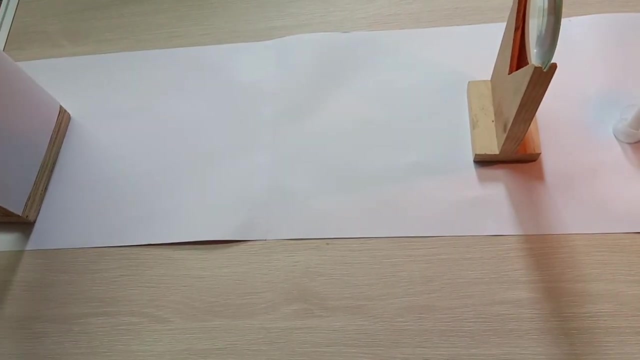 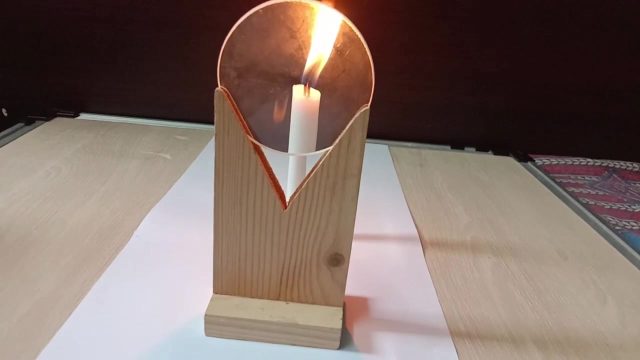 so we should be getting a virtual image, which we will not see in the video on the screen, because virtual images cannot be obtained on the screen. so i'm going to move the screen towards and away from the lens, but i am not getting the image. now, seeing through the lens, we are seeing that a candle and the flame is appearing. 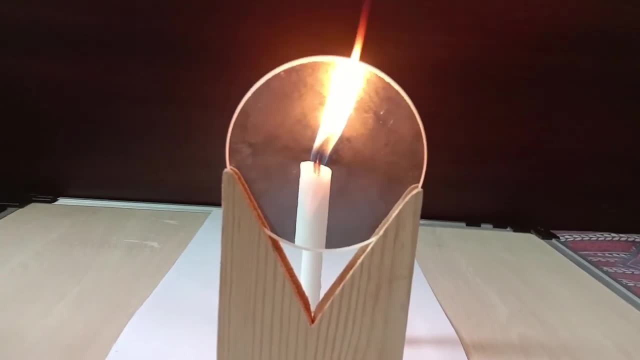 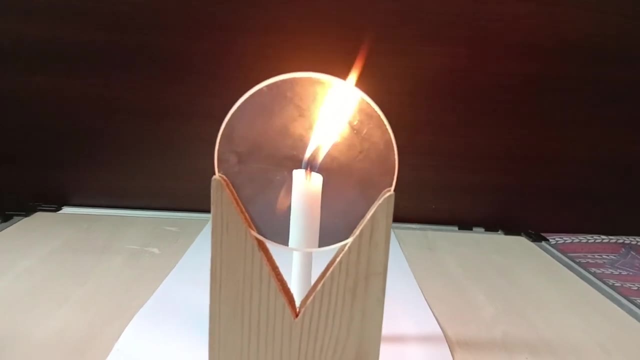 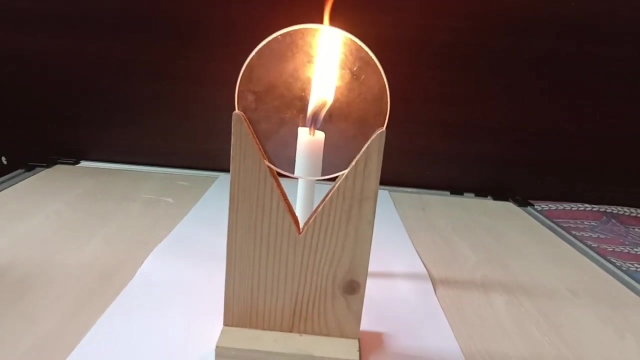 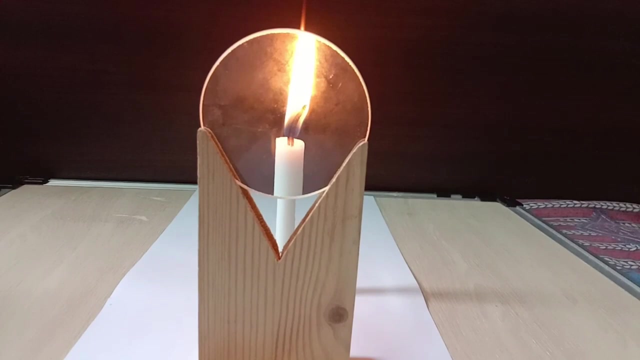 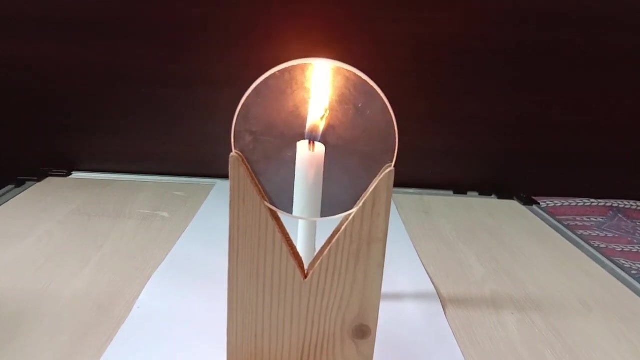 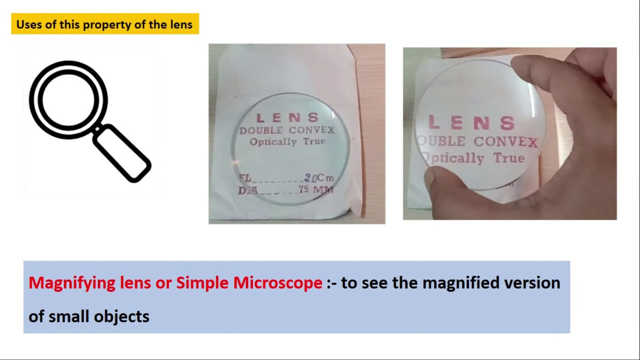 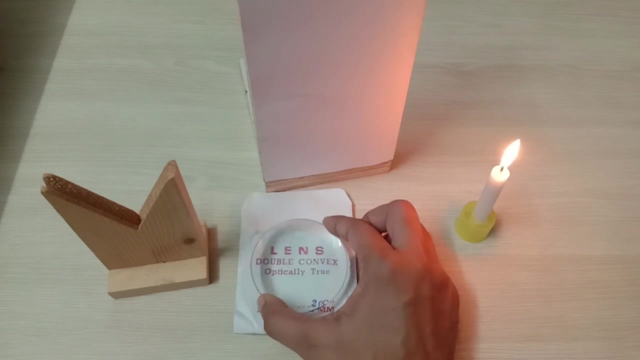 enlarged in the size. you can see the small part of the candle is visible under the lens. compared to that, we are getting the erect and enlarged image, or the magnified image. due to this property, the convex lenses are also referred as simple microscope. you can see that. 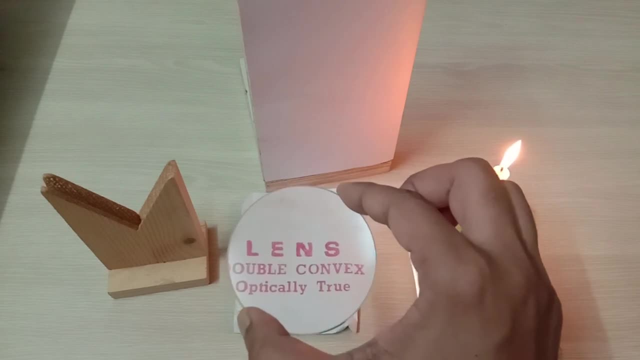 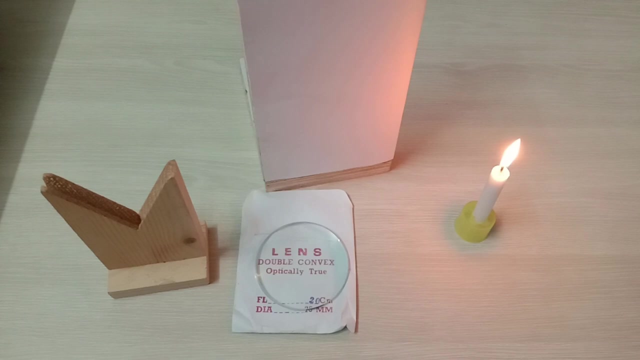 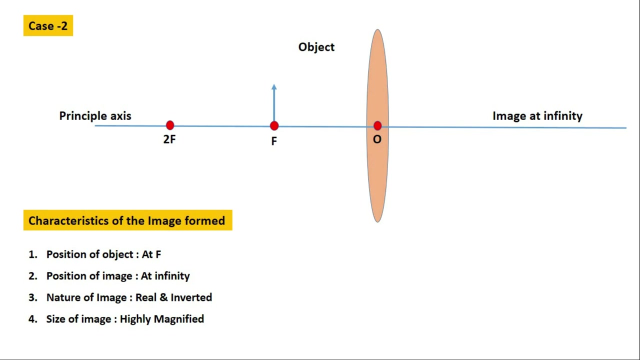 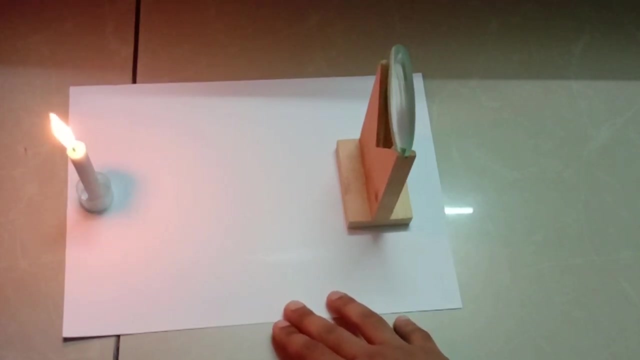 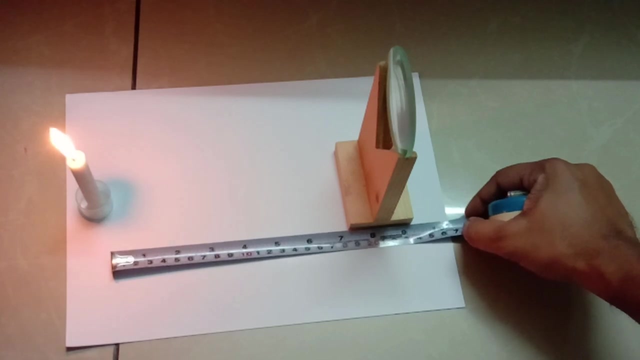 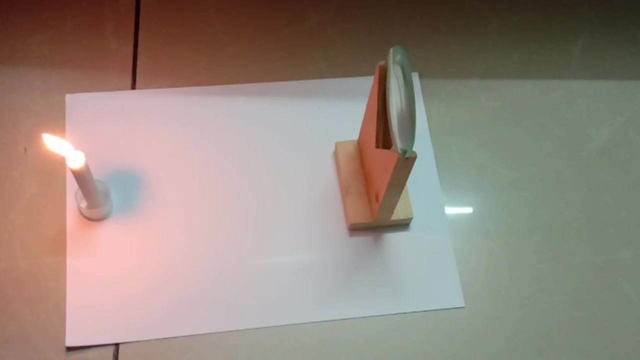 these letters are placed between optical center of the lens and the focus, so these letters are appearing enlarged here. the candle is placed at a distance of 20 centimeters away from the lens. that means the candle or the object is at focus. so we must get an image at infinity. now i want to 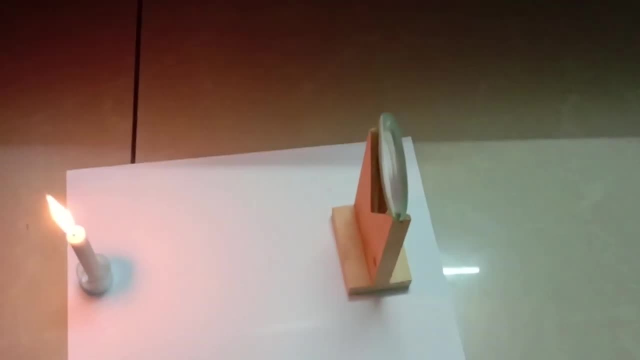 make sure that the object is at focus, so we must get an image at infinity now. i want to make sure that the object is at focus, so we must get an image at infinity now. i want to make sure that a point that any distance which is very large compared to the focal length can be considered as 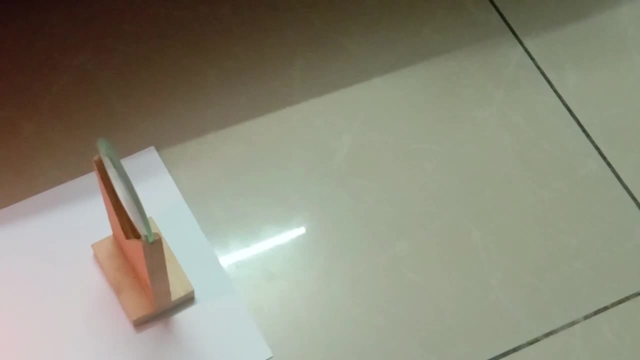 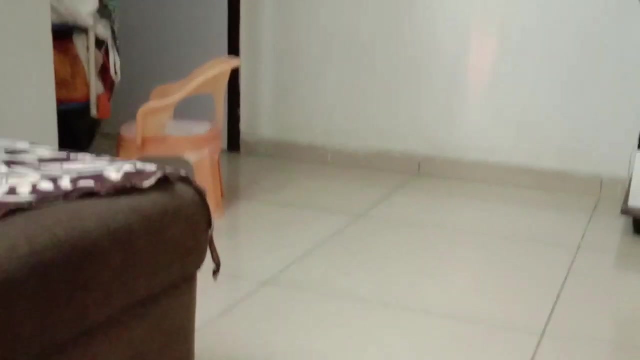 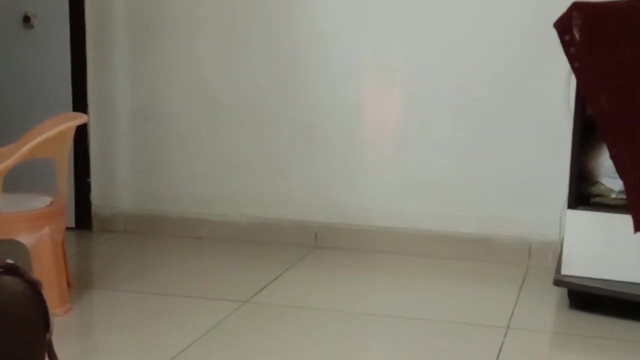 infinity. so you can see that the image is formed on the wall and the image is highly magnified, inverted and since it is obtained on the wall, wall behaves as the screen. so it's a real image and the wall is about 2.5 to 3 foot away from the lens. 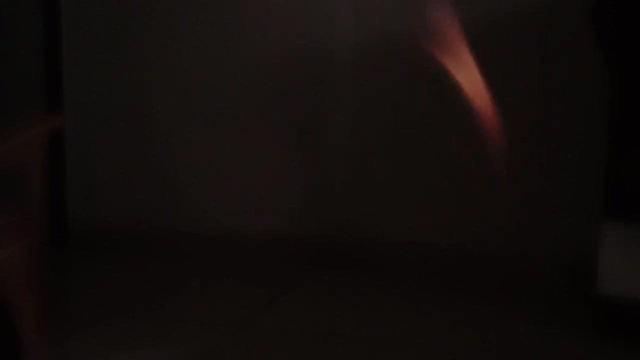 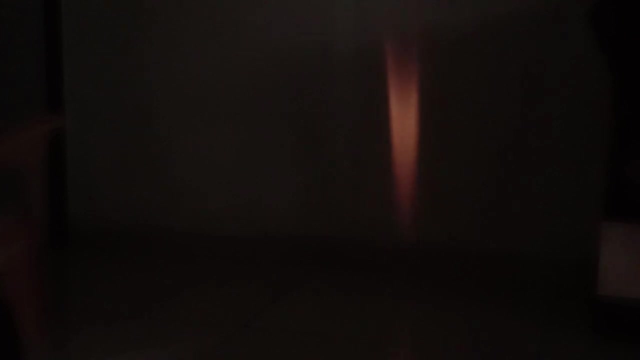 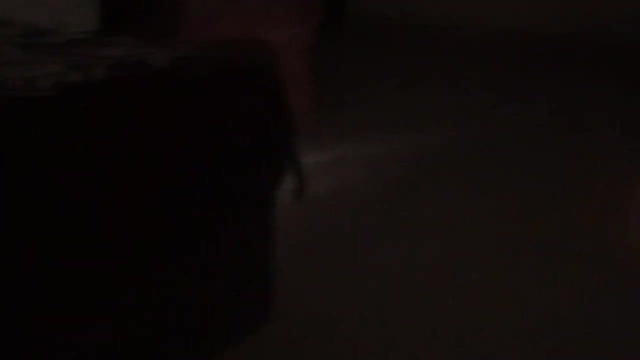 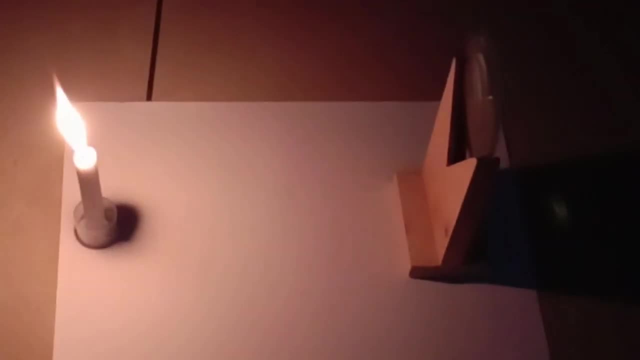 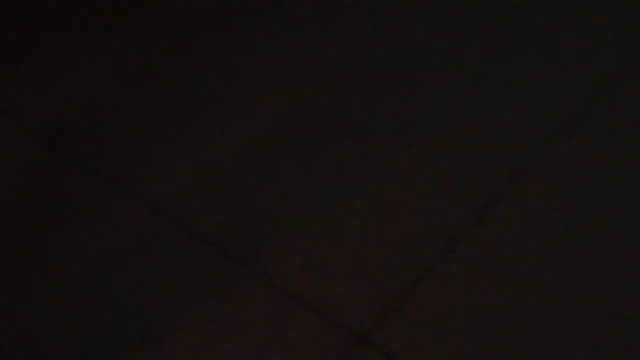 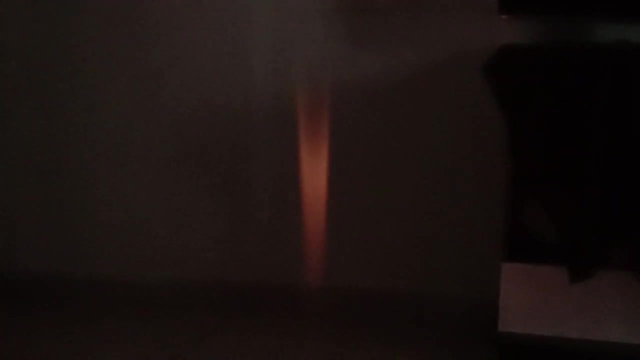 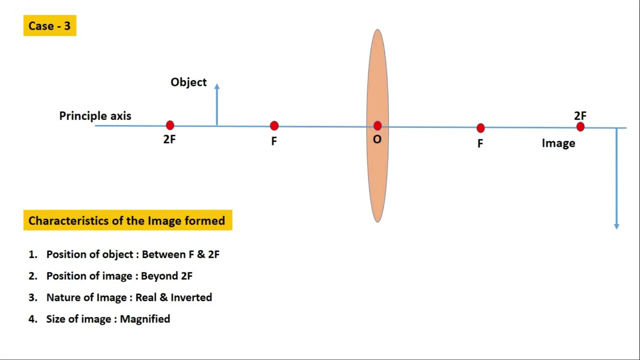 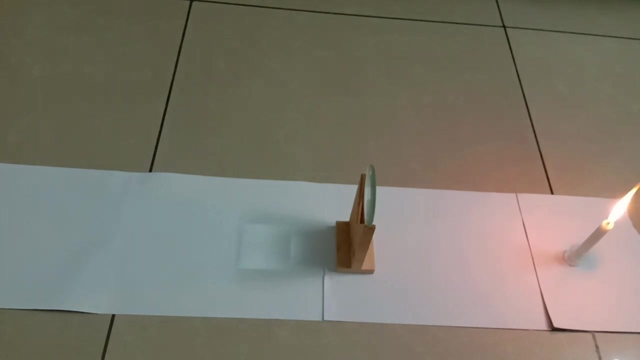 so this distance can be considered as an infinite distance. Thank you. Now, here the candle is placed at a distance of about 30 centimeters away from the lens, So this is the distance between 20 and 40. So this object is between f and 2f. 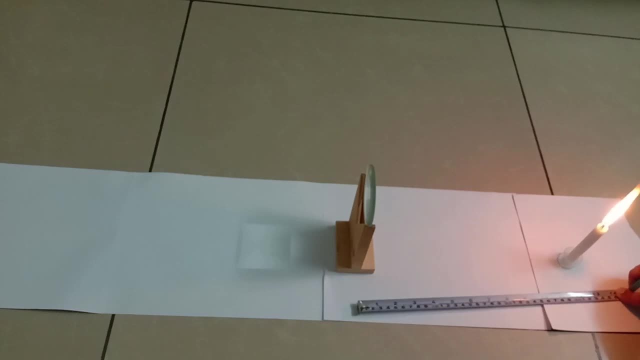 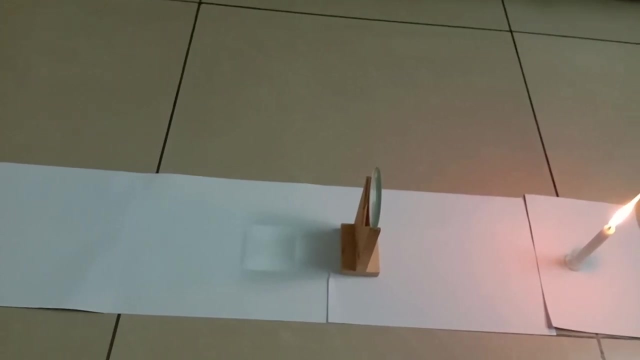 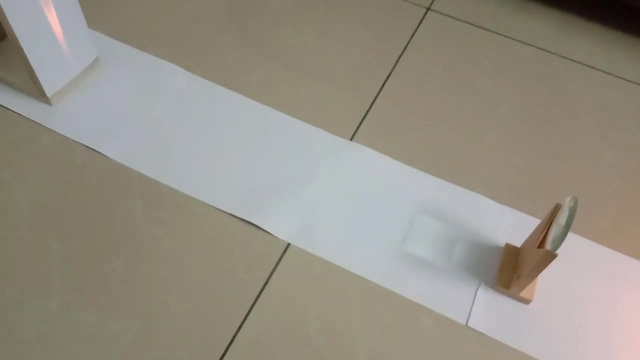 So we must get an image beyond 40 centimeters on the other side of the lens And it should be real, inverted and enlarged compared to the object. So I have already, I have already adjusted the screen and you can see that it's a real image because it is obtained on the screen. 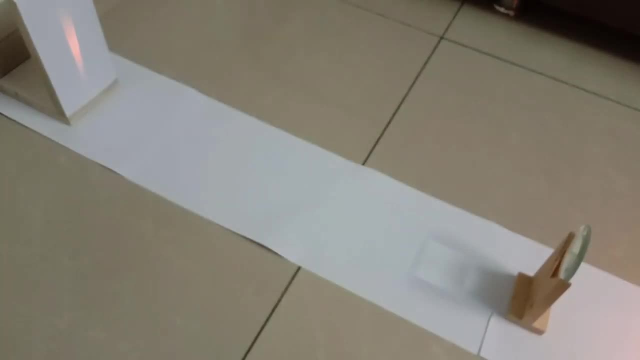 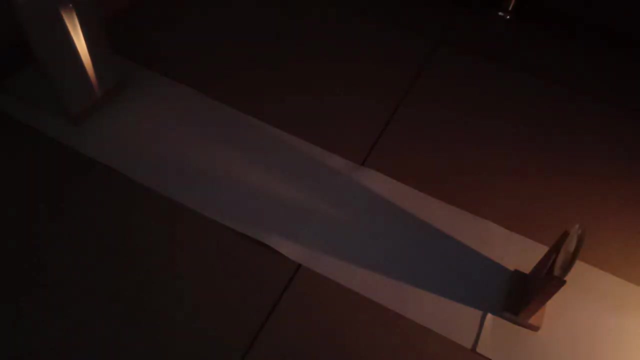 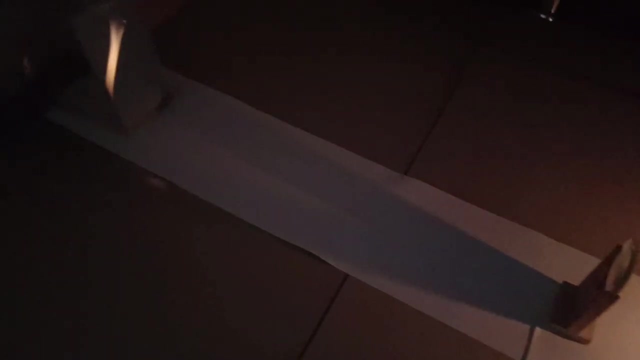 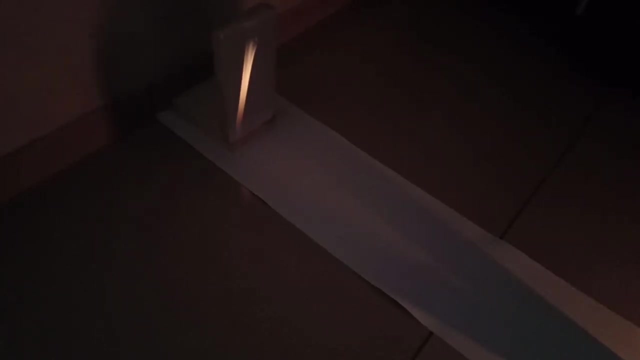 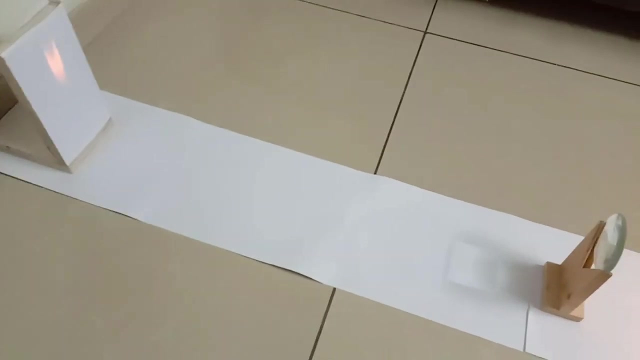 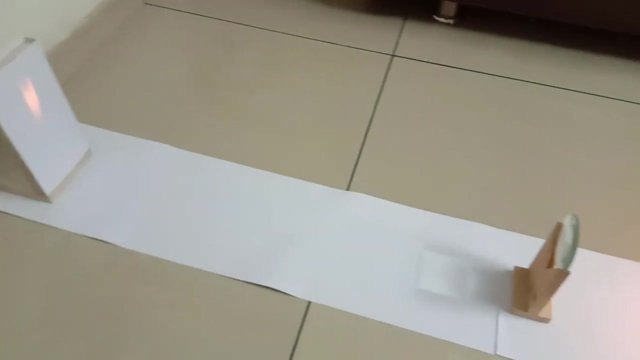 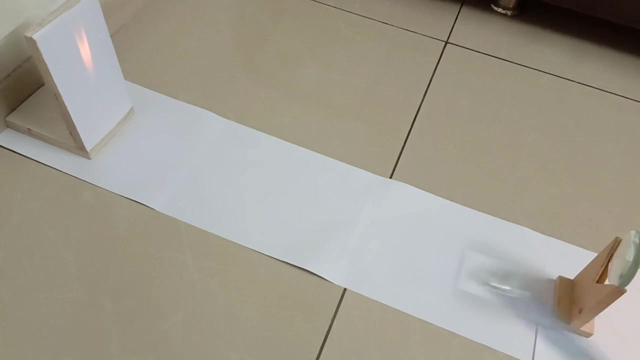 It is inverted as well as it is enlarged compared to the size of the original candle's flame. So I have already adjusted the screen and you can see that it is a real image compared to the size of the original candle's flame. So this is the distance between 20 and 40 centimeters. 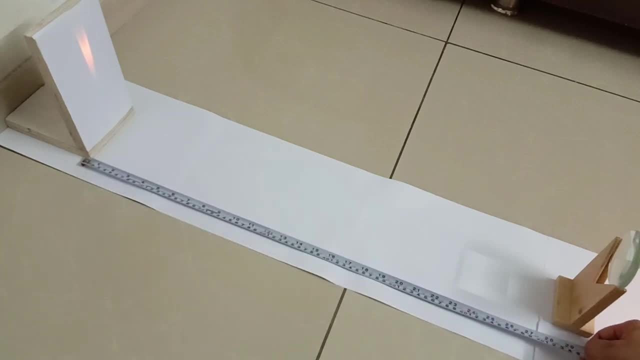 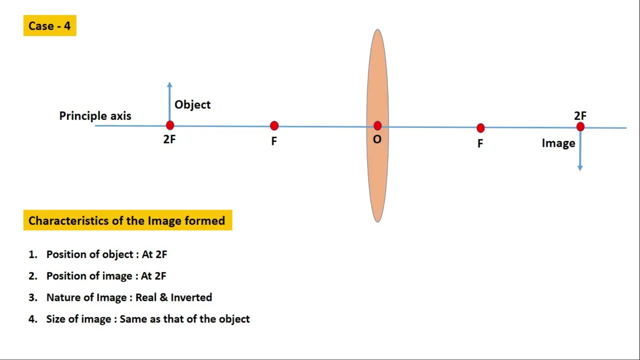 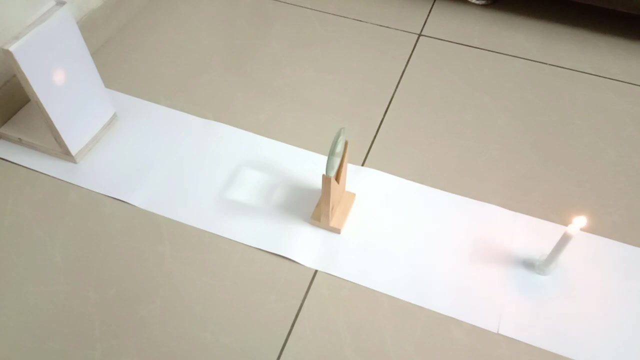 And the screen and the lens, which is the image distance is about 74 centimeters. Now here I am going to place the candle or the object at a distance of 40 centimeters away from the lens, So the object is exactly at 2f. 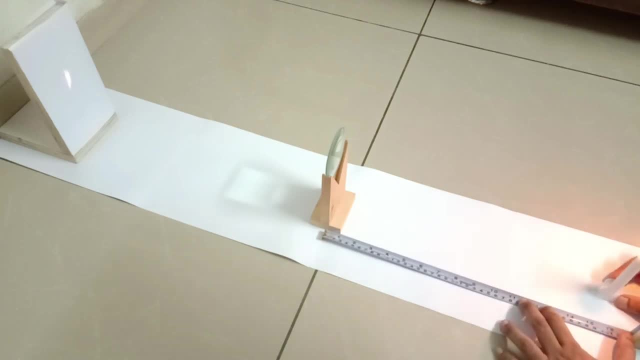 Because 2f is twice the focal length, Which is 40 centimeters away from the lens, And you can see that a real and inverted image of almost the same size as that of the candle's flame is obtained on the screen on the other side of the lens, and the screen is also at a distance of 40 centimeters from the lens. 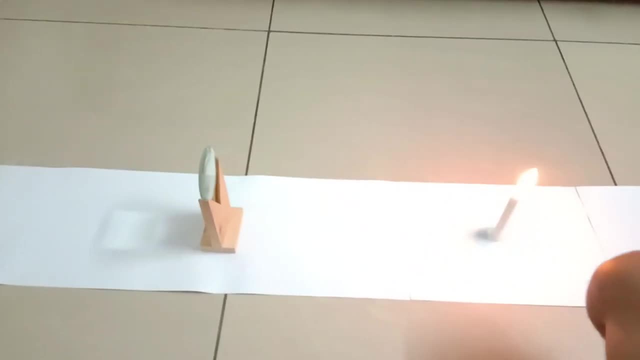 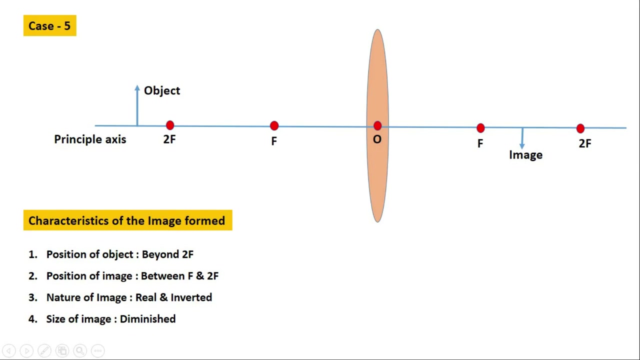 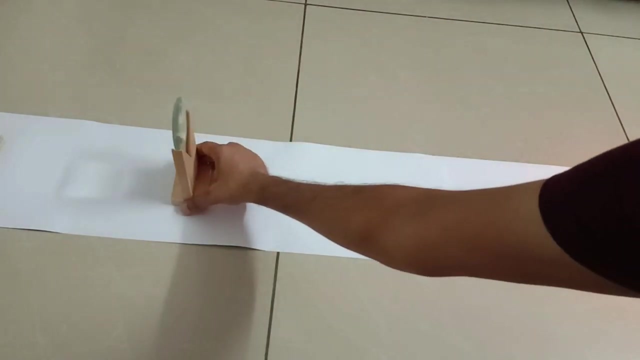 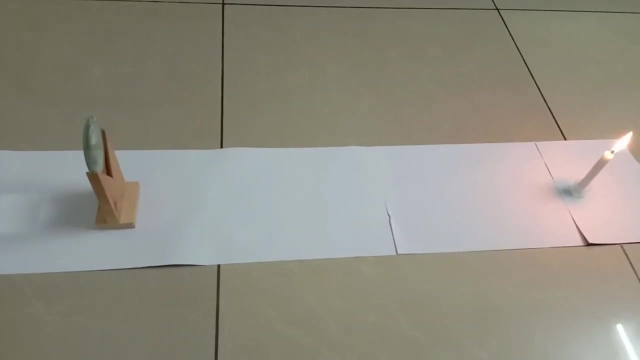 So the image distance is also 40 centimeters. So I am going to place the candle here And you can see that the blue light is also Puerto Rican light. Now, here I am going to place the candle At a distance of about 75 centimeters away from the lens.